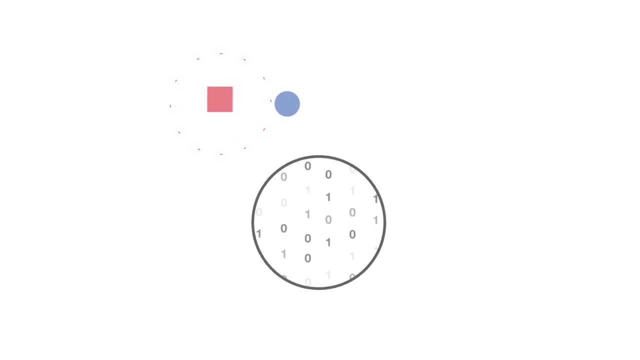 Being able to understand your business on a deeper level based on all of your data, and driving strategic decisions in real time is the essence of making big data work for you. From startups to Fortune 500 companies and worldwide public institutions- Amazon, Web Services- customers are running big data solutions in the cloud to gain actionable insights. 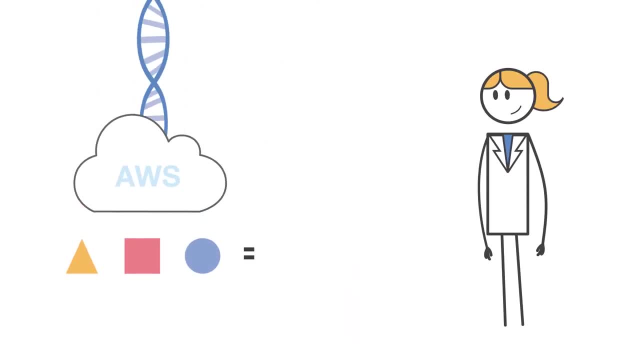 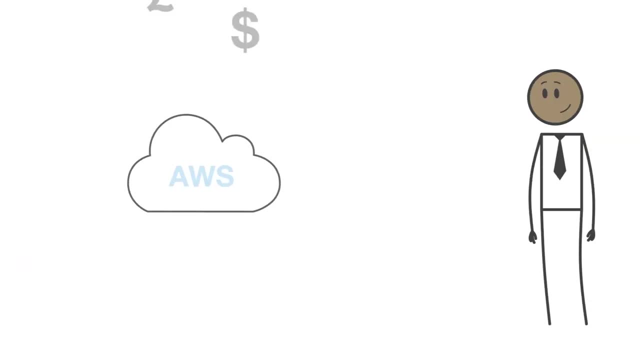 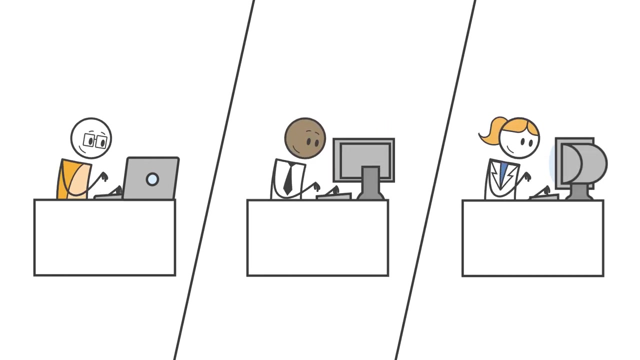 from their business data, Such as creating personalized medicine based on patient genetic information, delivering customized content to millions of users concurrently, or analyzing billions of financial transactions daily. AWS provides a self-service model where you can have on-demand availability of compute, networking and storage capacity at the speed. 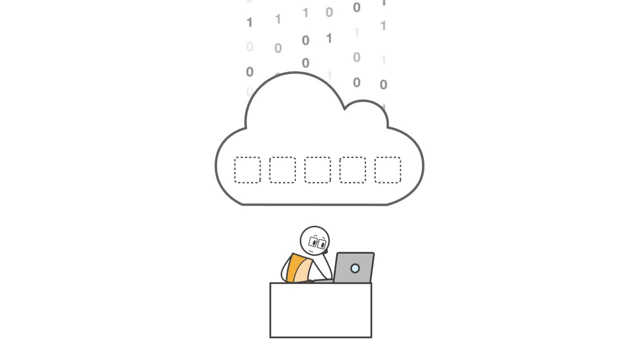 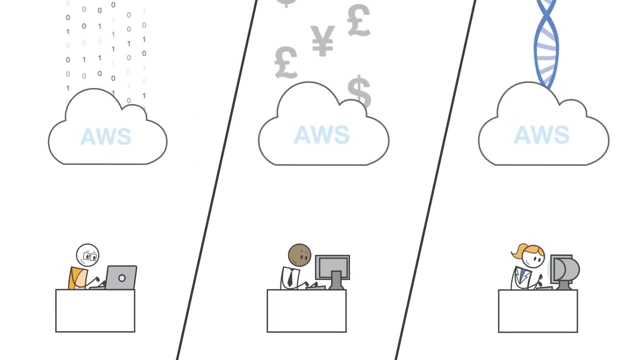 of a few mouse clicks. You have the flexibility to use AWS big data solutions, where much of the heavy lifting of provisioning, availability, durability, recovery and backup services are done for you, Or you can develop your own big data platform on Amazon Elastic Compute Cloud. 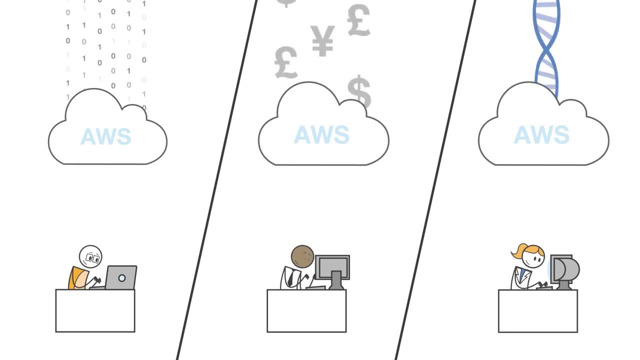 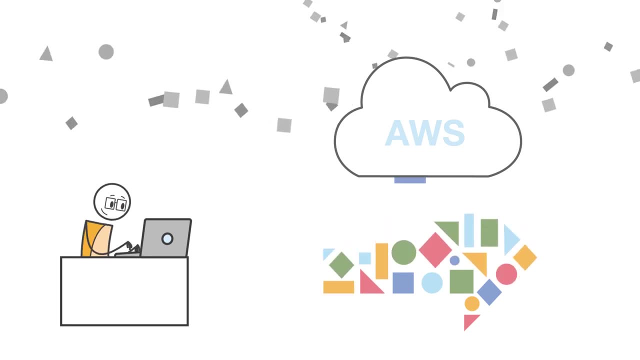 to meet your specific needs. The choice is yours. You can ingest data at any velocity from any number of sources, allowing you to process and analyze your data in near real time. Store any type of data, from unstructured data like documents and videos to structured data such as financial transactions and key performance indicators. 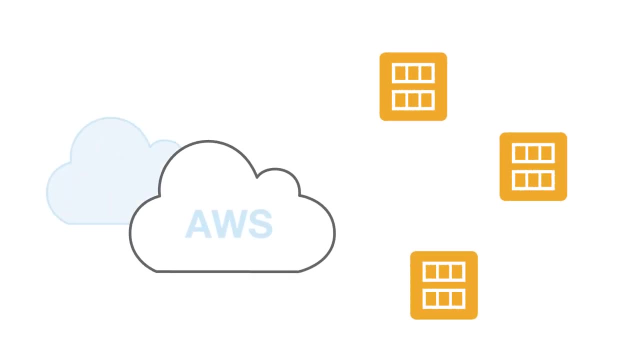 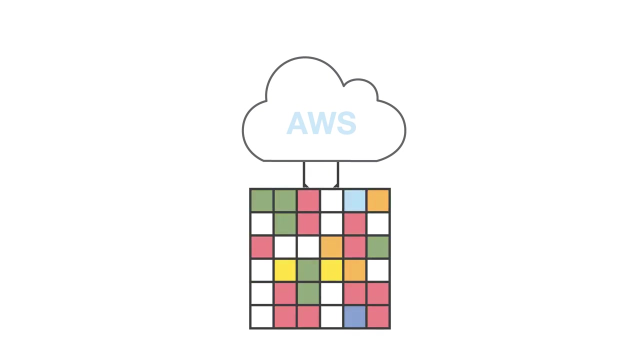 Analyze data at massive scale with up to thousands of servers working in parallel with software such as Hadoop, MapReduce, Hive, Pig, Spark or many of the emerging big data solutions. You can even create a data warehouse that you can resize dynamically. 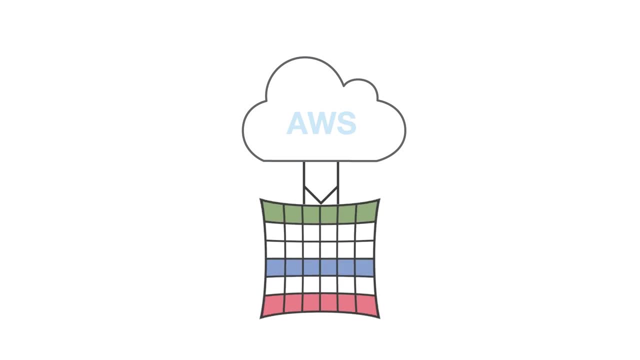 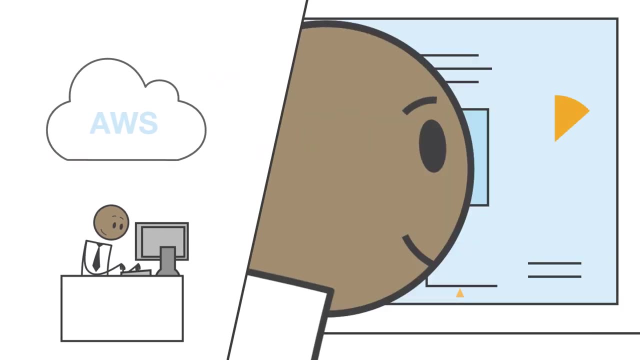 without downtime, from a few terabytes to multiple petabytes, as your needs change. Visualize and interpret your data with business intelligence and reporting tools that you're already familiar with. You can also create a data warehouse for your business intelligence and reporting tools that you're already familiar with. 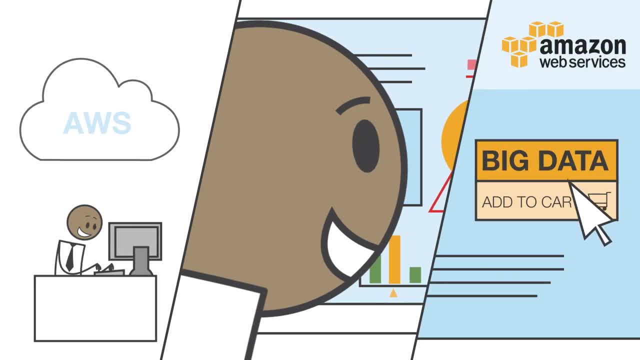 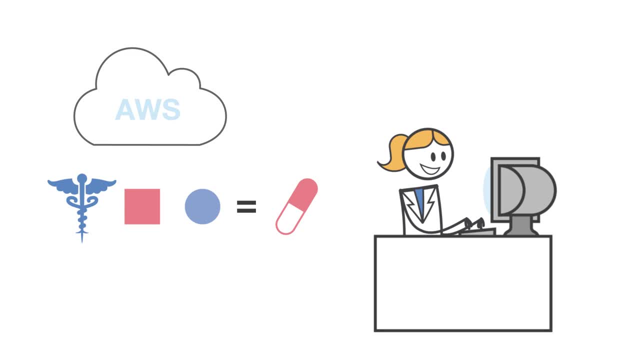 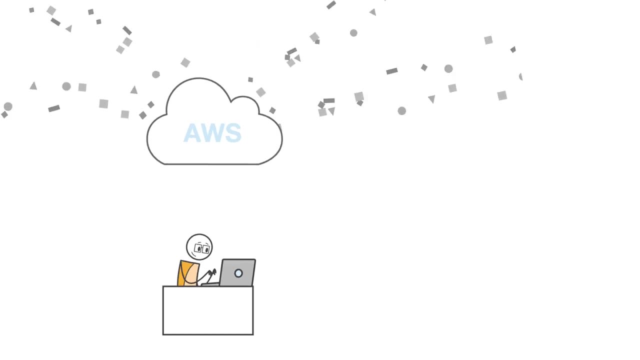 Or explore new solutions in the big data category on the AWS Marketplace. Success with big data comes from being able to iterate on your analysis, allowing you to focus on your business needs while not being held back by the cost and complexity of managing the IT infrastructure to collect, store, process and visualize your data.